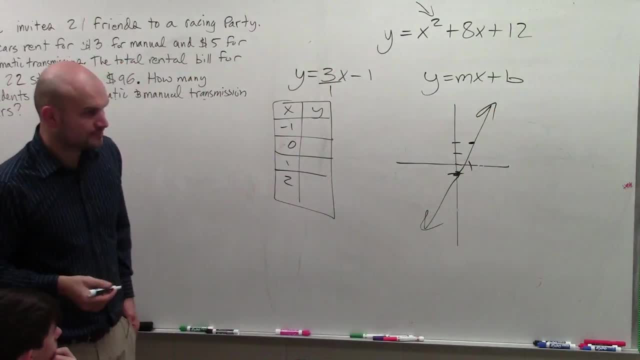 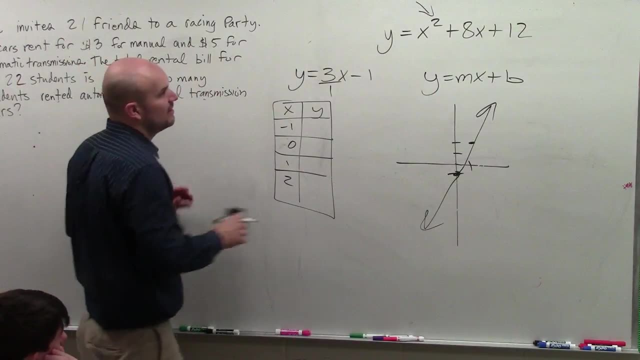 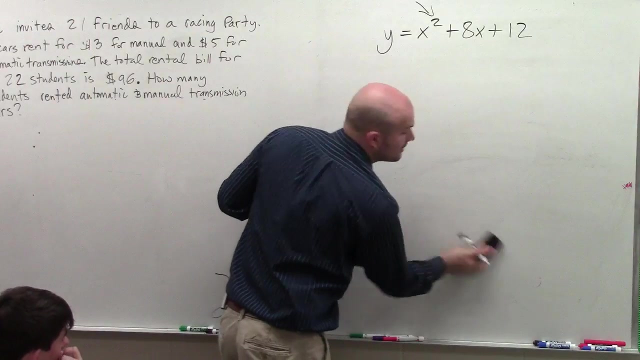 And then you could connect Right. It was pretty simple. Does everybody understand? Kind of with me, Okay? So, or if it was in standard form, we used the intercept method. Now for a quadratic. the shape: Yes, 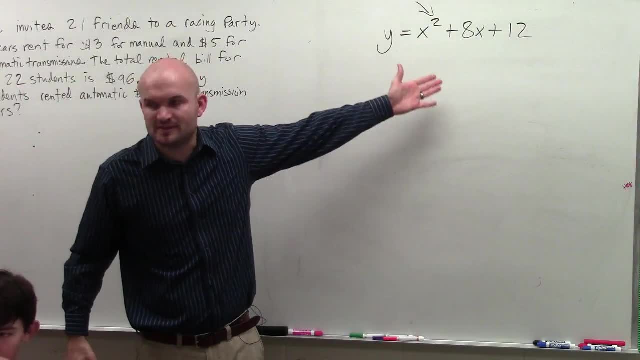 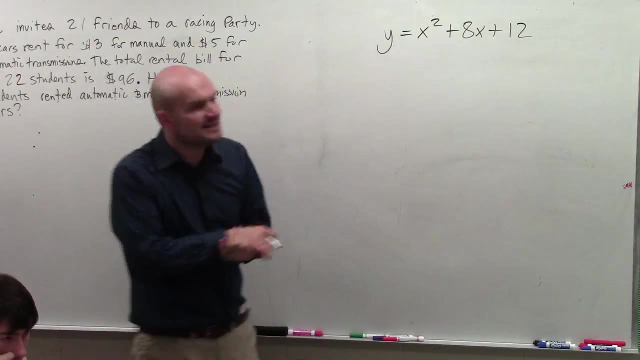 Yes, That was just a. that wasn't really a part of this problem. I'm going to do it again. I'm going to get into that. That was just a little forward And we're actually doing- Sorry, So, into graphing quadratics, what we're going to be doing is we're going to use the first method. 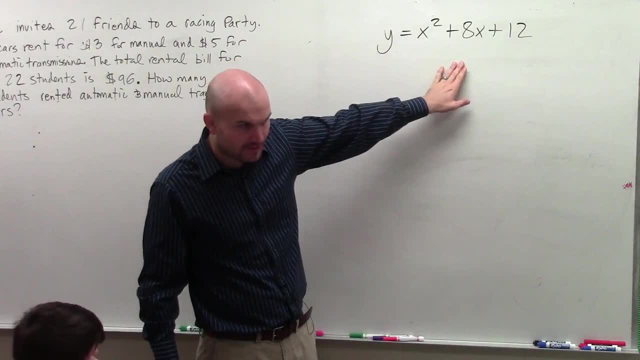 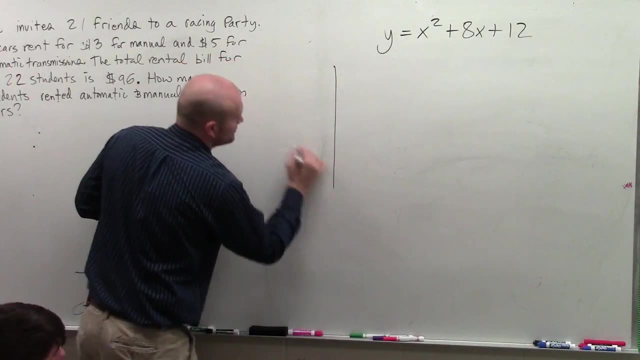 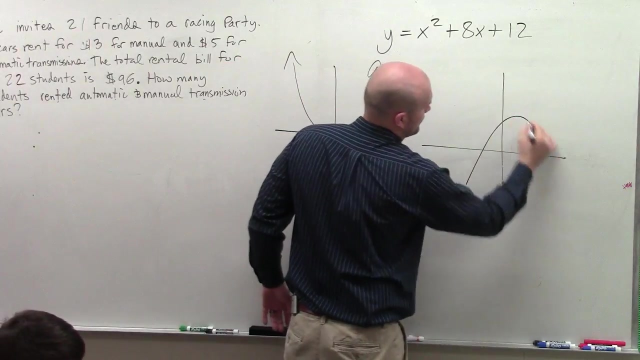 Okay, Which is when you have a quadratic in standard form. Now, a quadratic, the shape of the quadratic is not like a line, It is what we call a parabola, And a lot of times you can just relate it to a u. 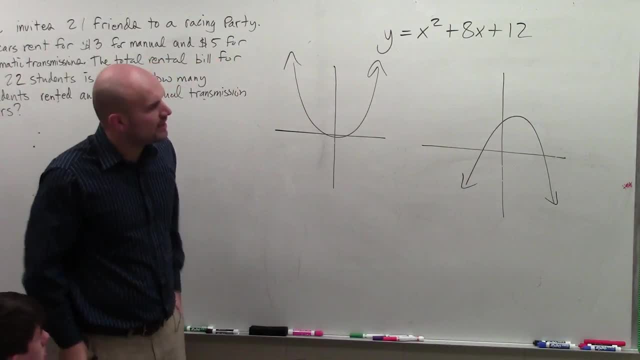 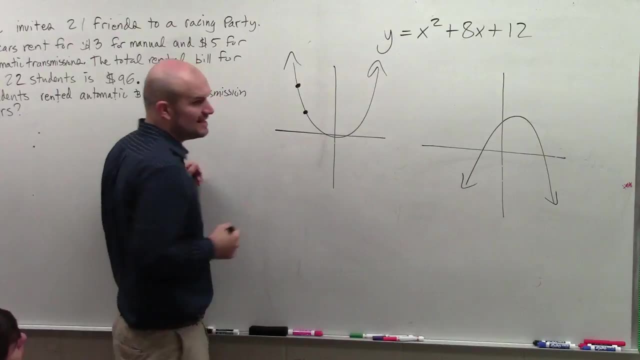 Okay. So the reason why I show you guys this, what you know some examples of a parabola look like, though, are because, if you just pick two points, does that tell you what the graph looks like? No, 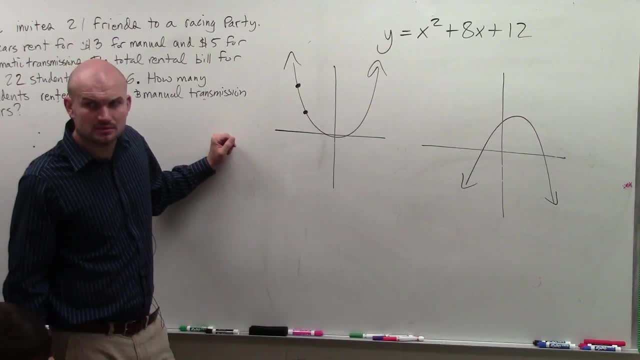 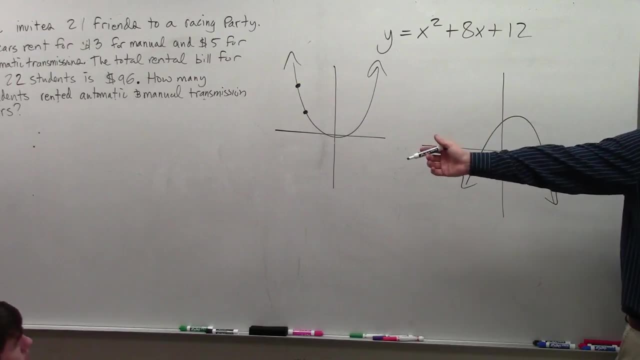 It doesn't right. Hey guys, girls, this is what I'm going over. This is the important thing I know. This is the important thing right here. So picking two points is not going to be enough, All right, 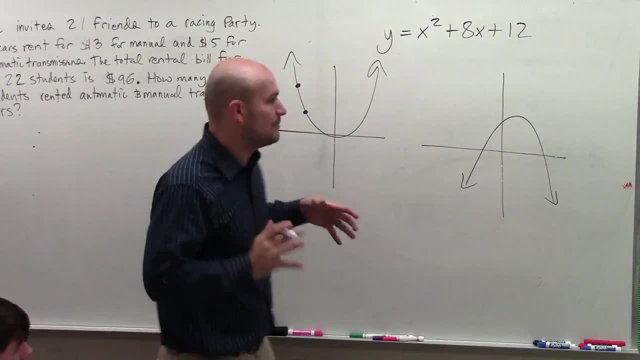 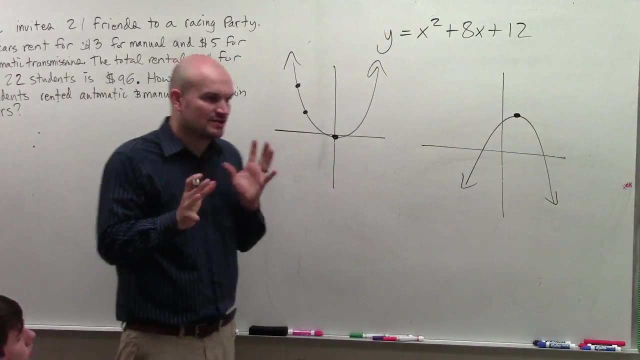 And there's another thing I want you guys to understand. I want you to make sure you write down: When we're dealing with quadratics, there's a very, very important point. There's actually two. there's two kind of important characteristics: the minimum or the maximum. 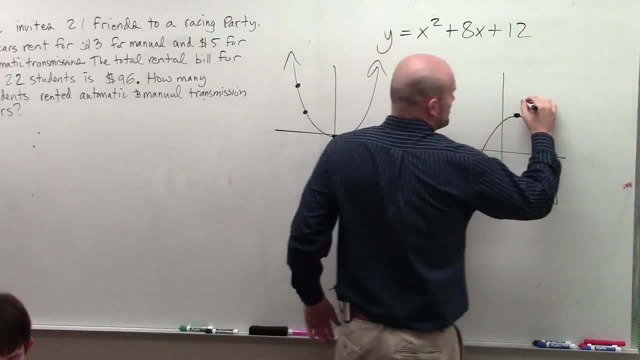 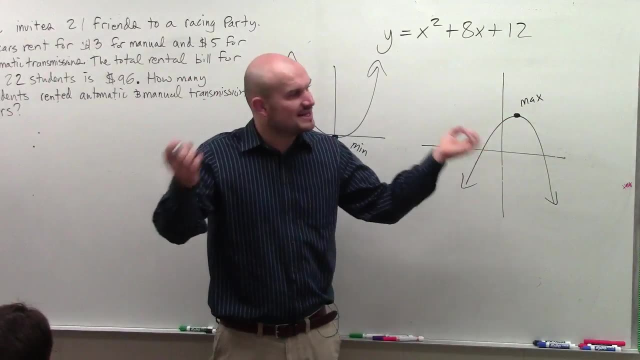 And whenever you have the min or the maximum point. do you guys see how that's like the minimum point of this parabola right here? And that's the maximum point. Any point that it takes the minimum or the maximum is what we call our vertex. 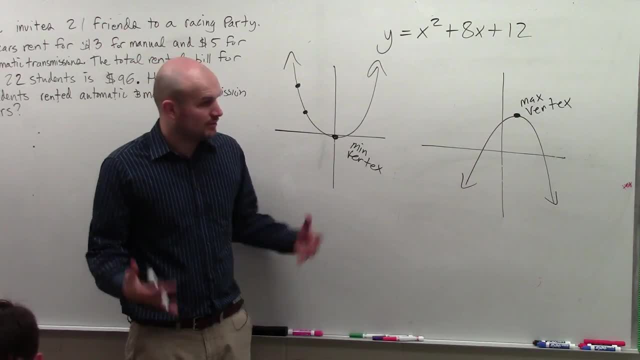 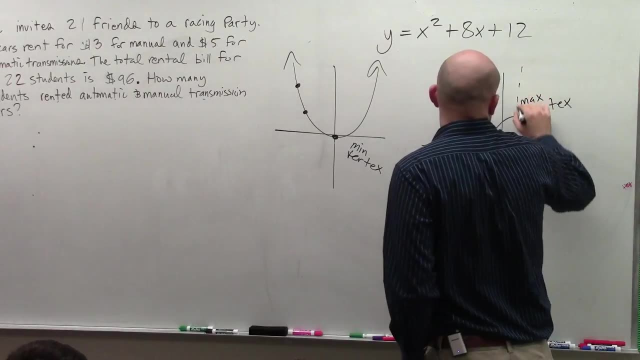 Okay. So you're going to want to make sure you understand that. The next thing is: through the vertex, there is a line of symmetry. So I'm not going to be the best drawer here, but if you guys remember, in geometry 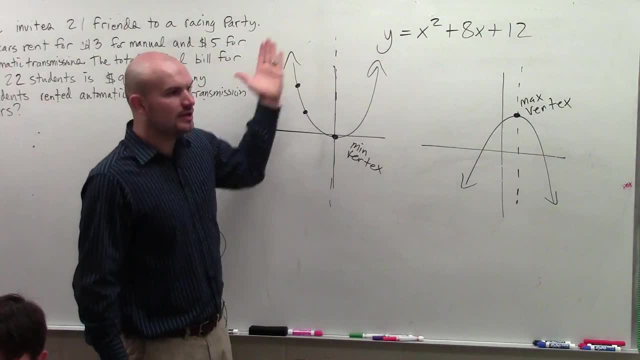 a line of symmetry is a line about where which you can flip your graph over, and it's going to be symmetrical with: Do you guys see that, If you were to kind of take that and fold it over that dotted line, Okay, 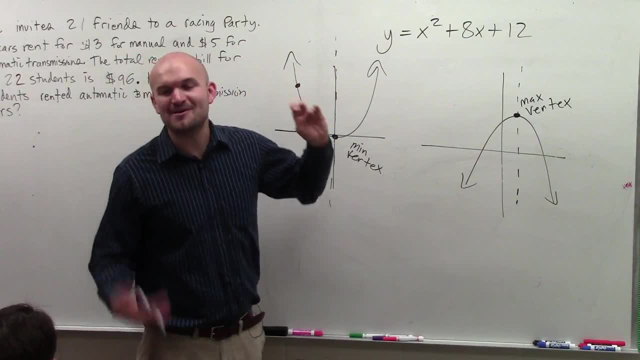 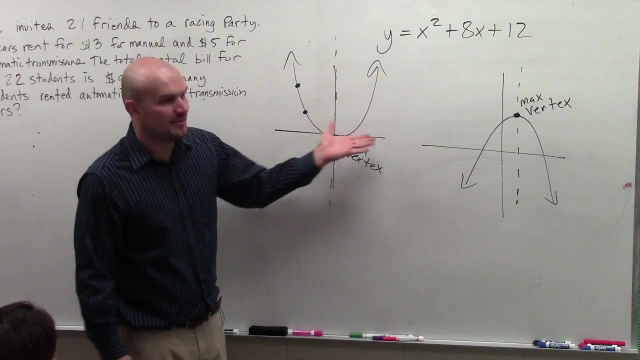 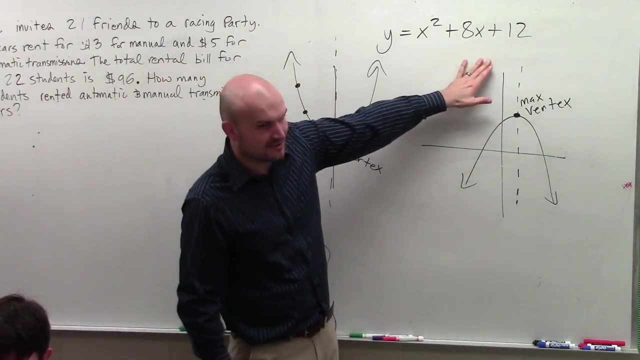 Right, Elizabeth, from geometry. Right, Right, Okay, Okay, Okay, Right. No, I'm just saying from remembering from geometry: Okay, Does everybody see what we have here? Yes, Okay. So when we're getting into graphing now what we're going to do when we're graphing, 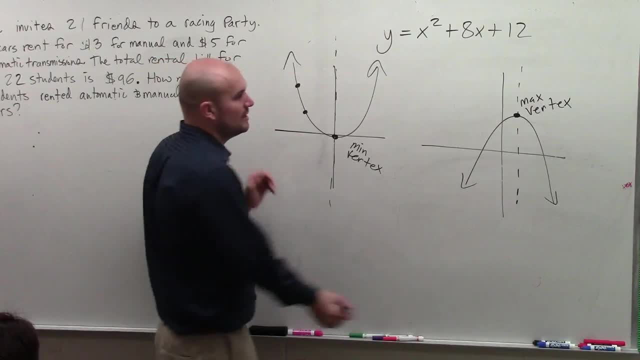 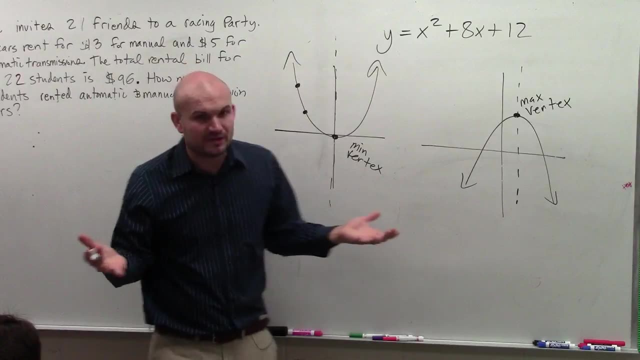 a night when we graph a quadratic, what I'm going to expect you guys to do is the first thing we're going to do is find the vertex. We're going to find that point and we're going to plot that point. Remember, when we graphed linear equations, the first thing we did was graph the y and. 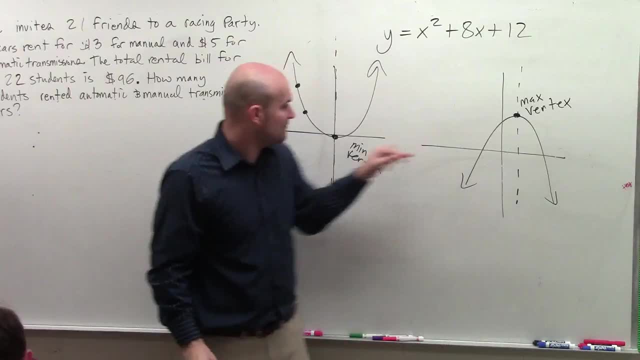 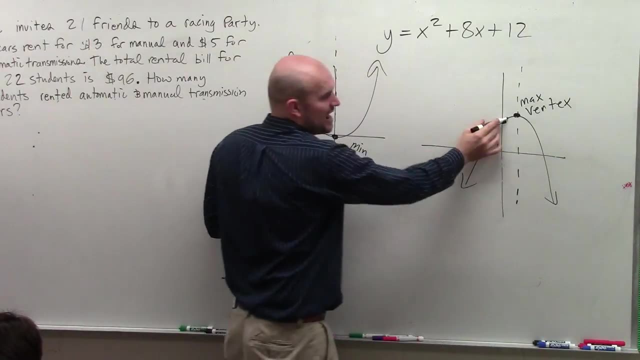 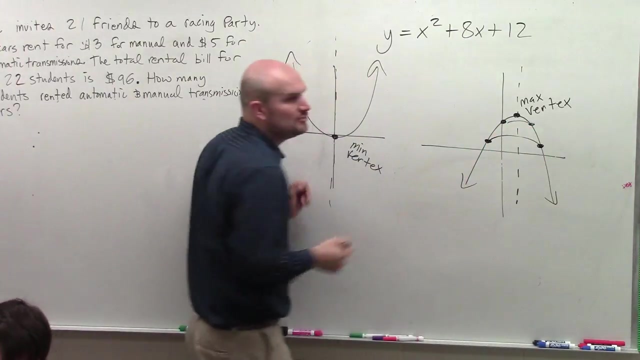 y intercept. Right Now, the first thing we're going to do is graph the vertex. Okay, Then what we're going to do is pick two points to graph, either to the left or to the right of the vertex, And once you know two points, can you now use those other two points or the line of 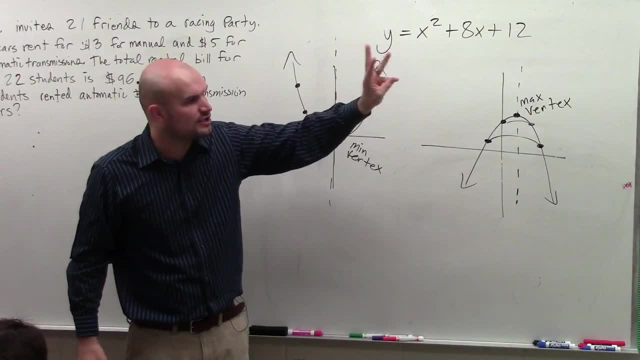 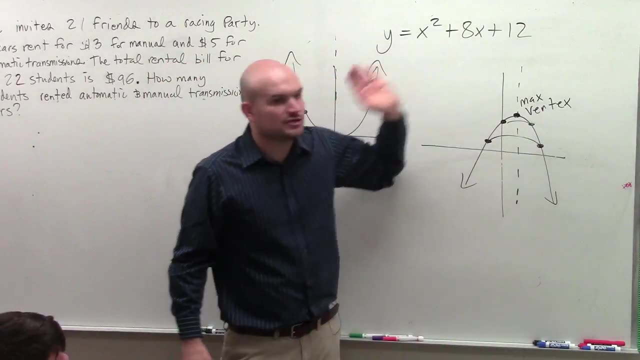 symmetry to reflect over there. So really, ladies and gentlemen, all we're going to do is now, instead of two points, we're now going to add it up to three points that we're going to graph, and then you're just going to reflect those other two points. 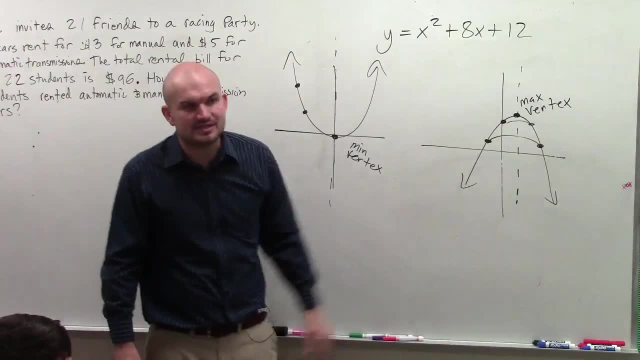 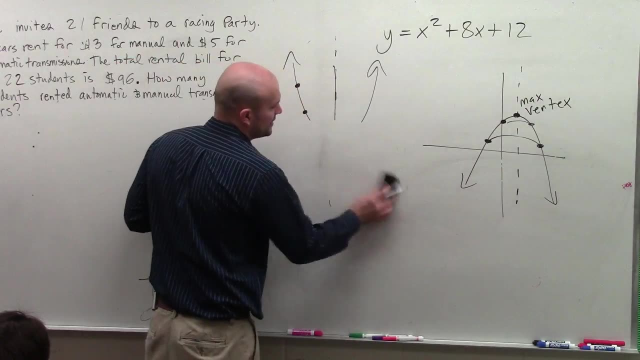 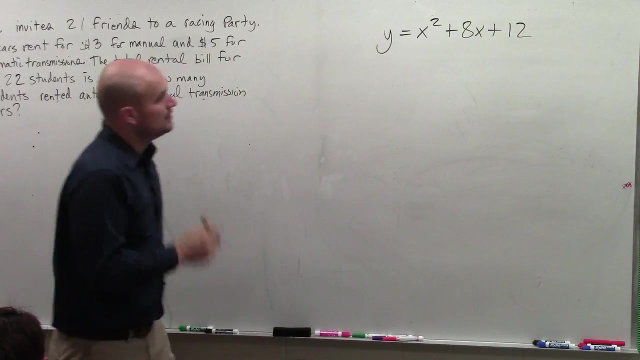 Two points across the line of symmetry, and then you have five points that you can use to graph this. Make sense? All right? Well, let's go ahead and see what we're going to do here. So how do you find the vertex? 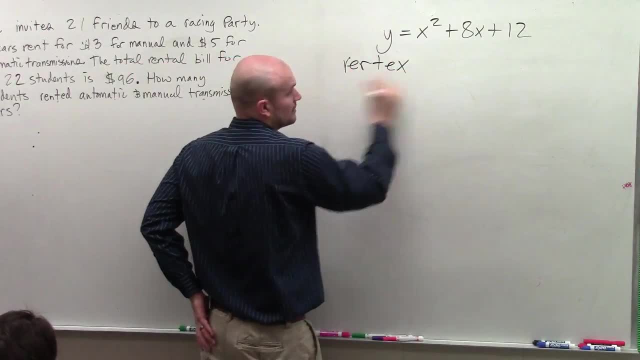 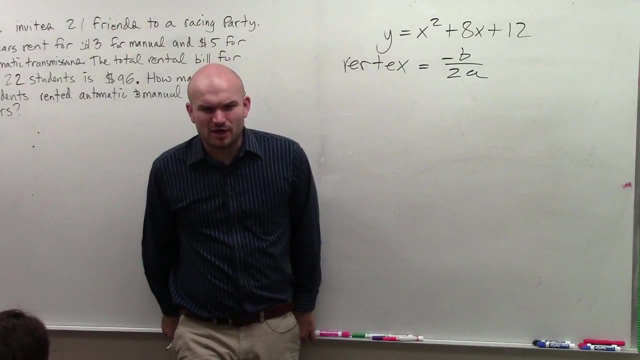 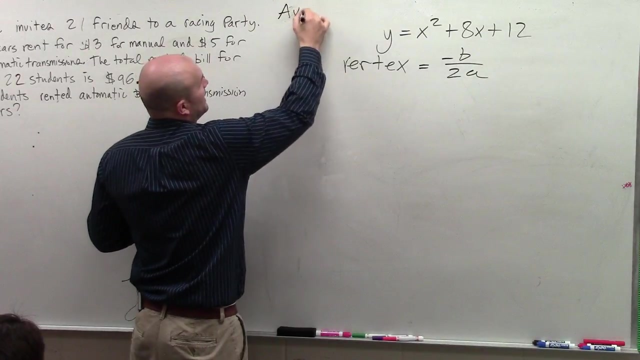 So the vertex, the formula for the vertex, equals opposite of b divided by 2a. And some of you might say, okay, where did you get? Where did you get the a and the b? Well, if you guys remember, ax plus by equals c. 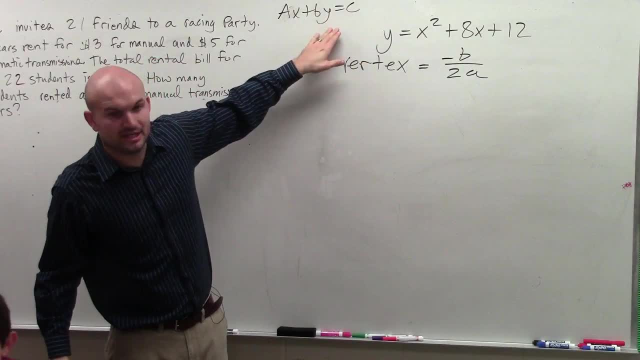 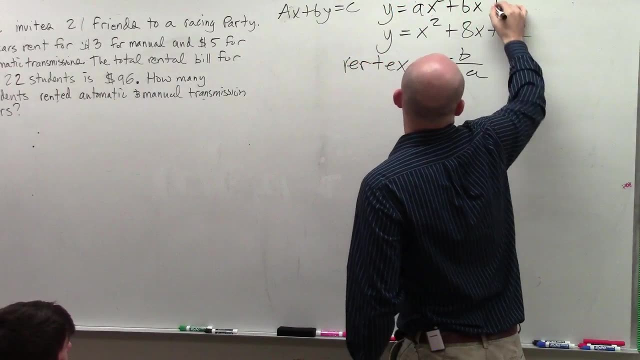 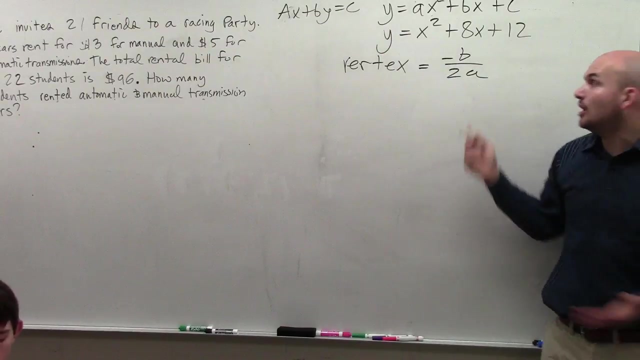 That was what we wrote, for. That was standard form of a linear equation, right? So standard form for a quadratic equation looks like this: Do you guys see that? That is your standard form for your equation. So now all I got to do actually kind of my steps that I like to do- 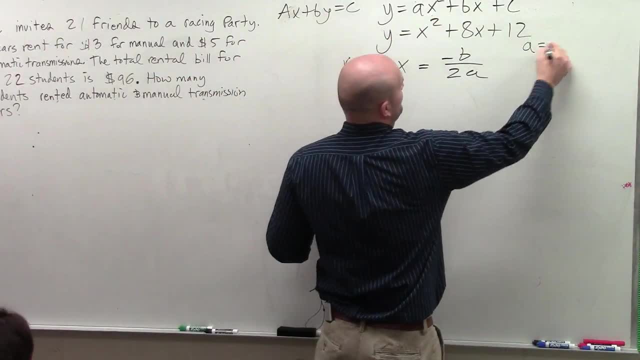 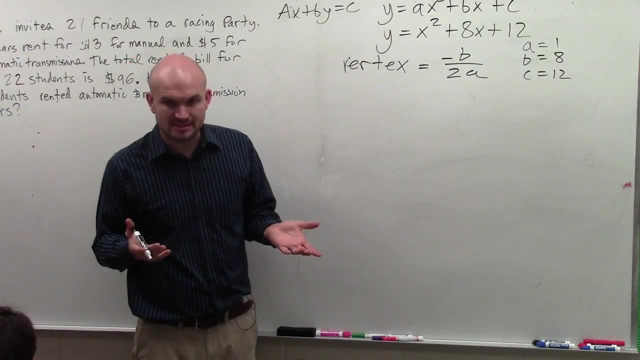 Is, first thing, identify my a, b and my c. A equals 1., B equals 8.. C equals 12.. Does everybody see how I labeled my a, b and c? Yes, Okay, Now I'm just going to evaluate to find my vertex. 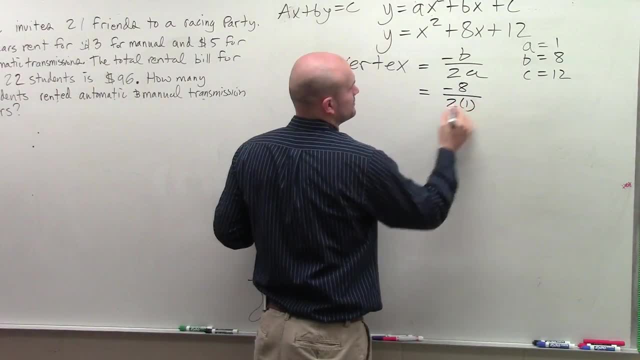 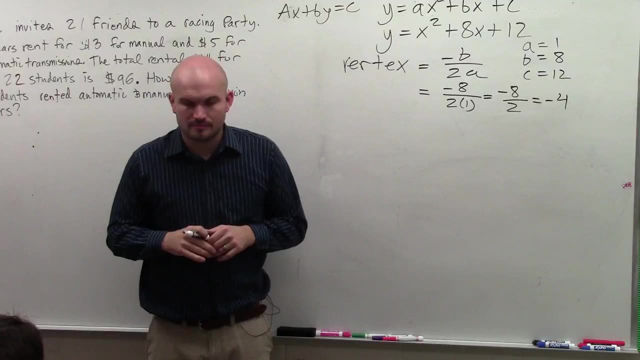 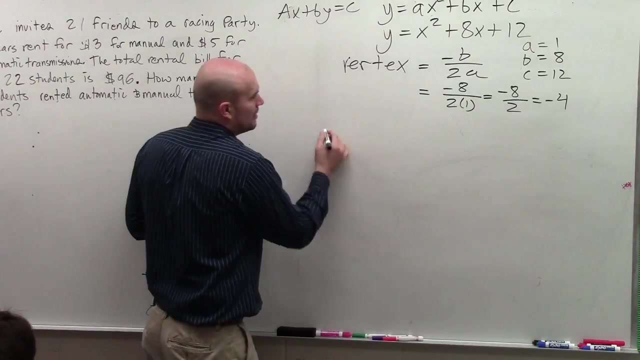 So I do opposite of 8 divided by 2 times 1,, which equals negative, 8 divided by 2, which equals negative 4.. Everybody follow me, Yeah, Yeah, Yeah, Yeah. So now I don't know my vertex though. 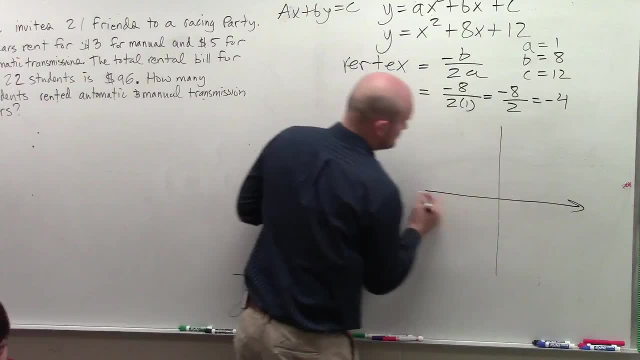 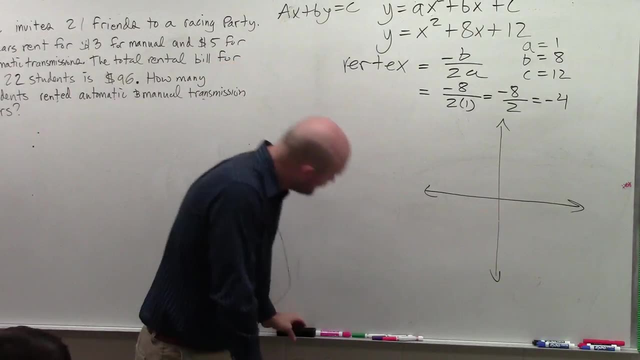 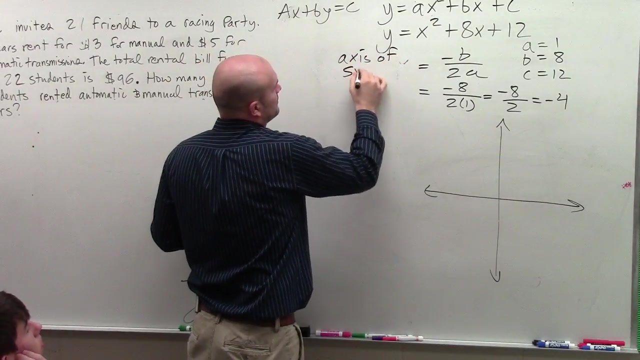 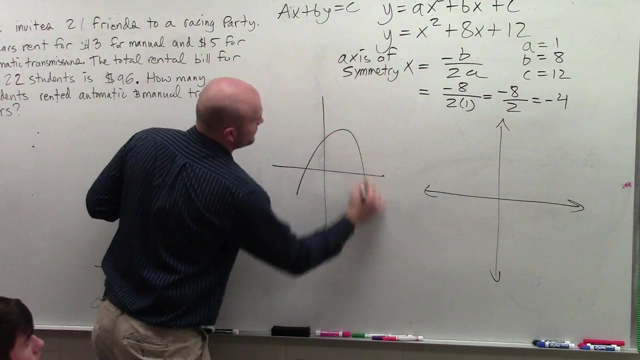 I don't know what that point is. All I know is that point is shoot. I'm sorry, That's not the vertex. That's your axis of symmetry. Sorry If you guys remember when I did this graph. Okay. 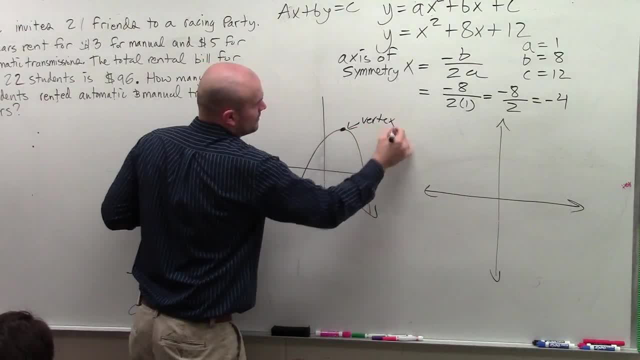 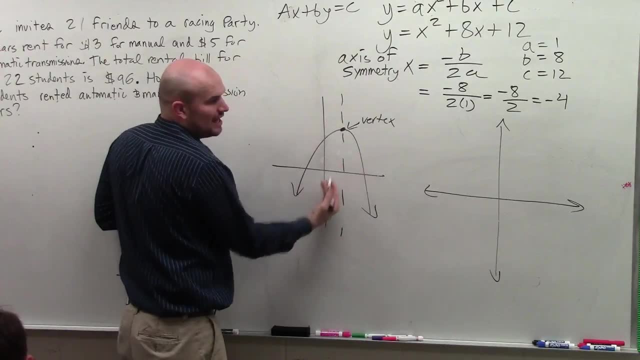 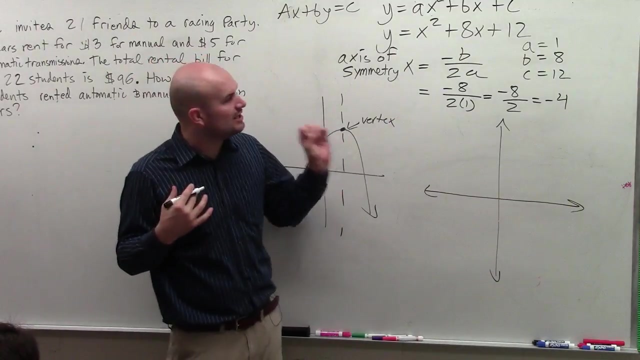 remember here was the vertex right. remember the axis of symmetry goes through the vertex right. notice that's a vertical line. vertical lines are in the form of x equals, correct? so I'm sorry I just been over break. I I missed stoke my thing. so, Elizabeth, when I'm describing this, your vert, your horizontal line, is: 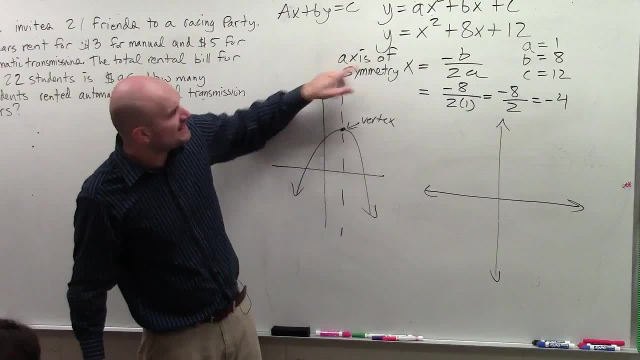 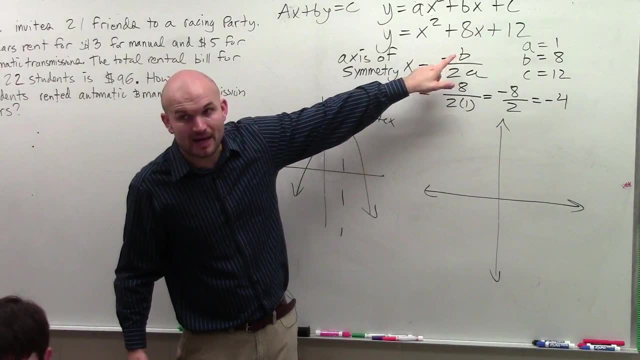 your vertex. so the first thing you want to do is not find the vertex, but we want to find the axis of symmetry, which is the x-coordinate of my vertex. so I still do opposite of B divided by 2a. I do opposite of B divided by 2a and I get x. 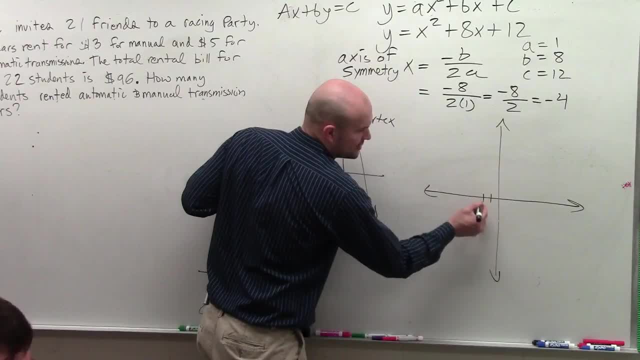 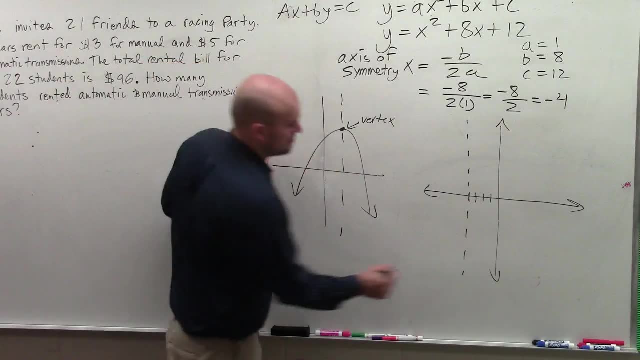 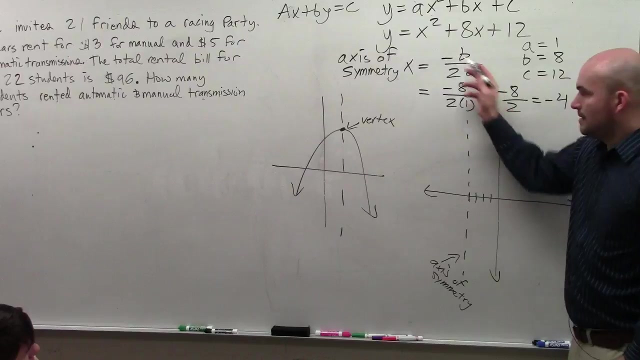 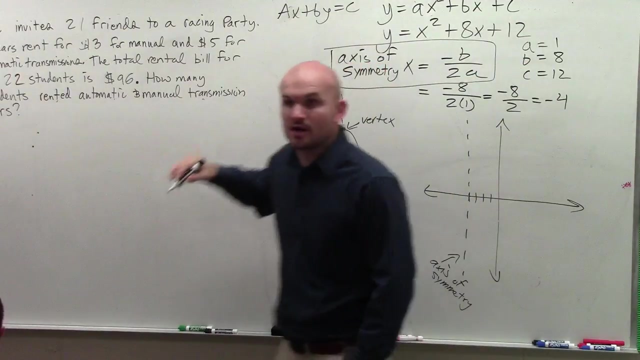 equals negative 4. therefore, I go to next. equals negative 4, 1, 2, 3, 4 and I draw my axis of symmetry. does everybody see that axis? symmetry always equals x, equals opposite of B divided by 2a. yes, you're gonna want to have that memorized because you are. 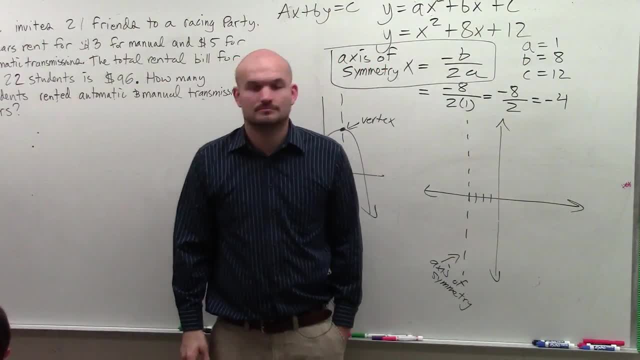 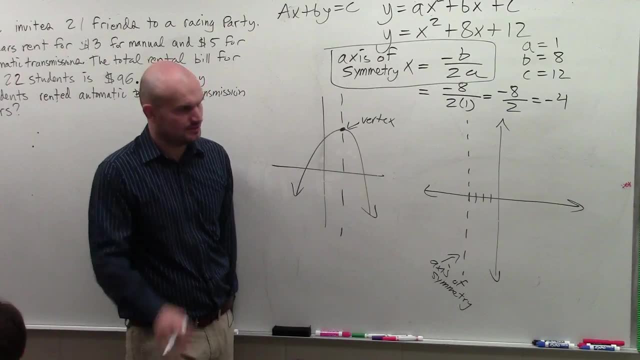 gonna have to know how to do that. my apologies I it's been a long break, but does everybody see that and understand it, mas amenos? okay now, where does this point, though, lie on this graph? well, okay now, where does this point, though, lie on this graph? well, 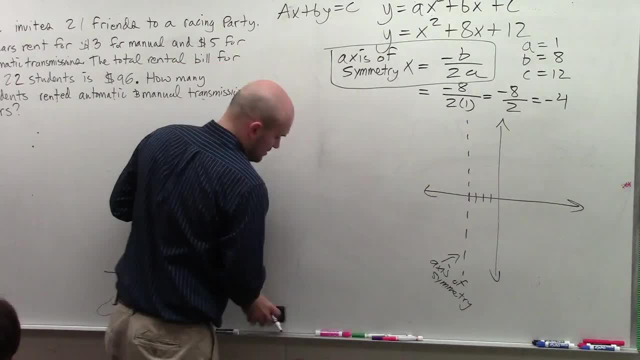 where does this point, though, lie on this graph? well, where does this point, though, lie on this graph? well, to do that, you're gonna have to do that. you're gonna have to do that, you're gonna have to go back to your table. so, X, Y, we know that. our 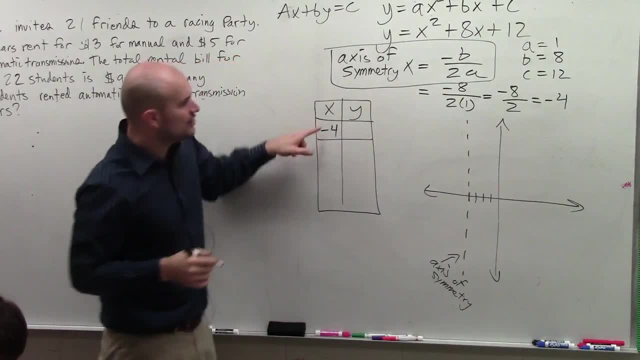 to go back to your table, so X- Y. we know that our to go back to your table, so X- Y. we know that our coordinate is negative 4 right coordinate is negative 4 right coordinate is negative 4 right. so to find the y-coordinate we got to. 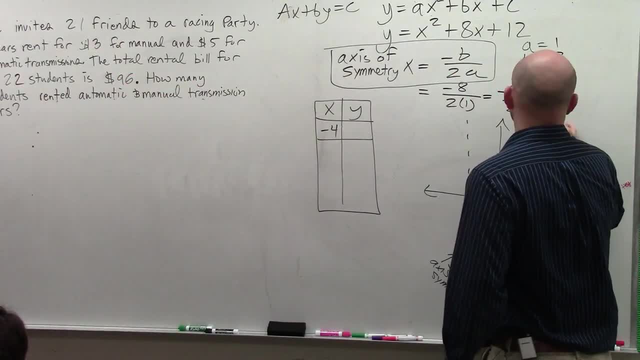 so to find the y-coordinate, we got to. so to find the y-coordinate, we got to plug negative 4 in for X. so I do y plug negative 4 in for X. so I do y plug negative 4 in for X. so I do: y equals negative 4 squared plus 8 times. 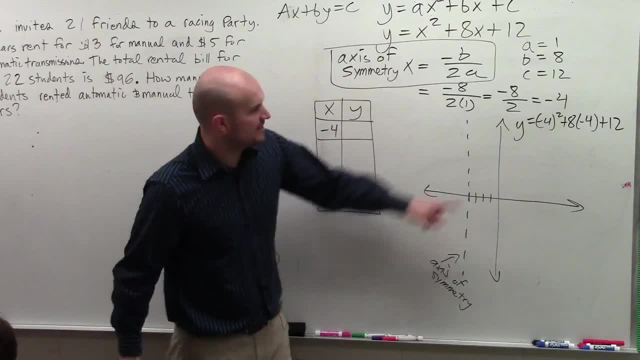 equals negative 4 squared plus 8 times. equals negative 4 squared plus 8 times negative 4 plus 12. does everybody see negative 4 plus 12? does everybody see what I did there? I took my x-coordinate and I plugged it into my equation to find my y-coordinate. 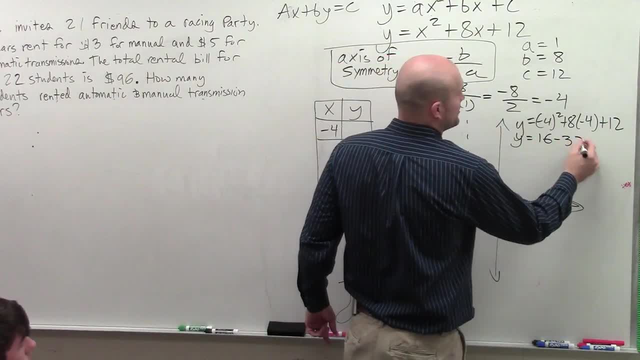 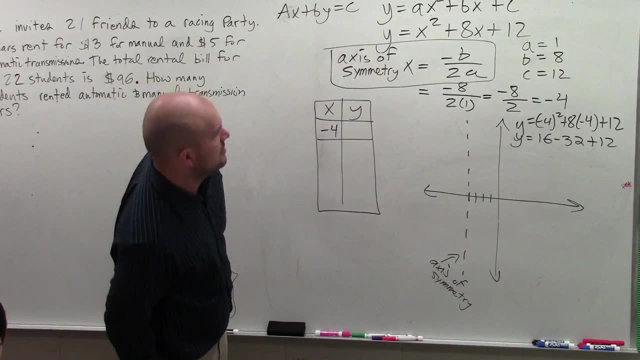 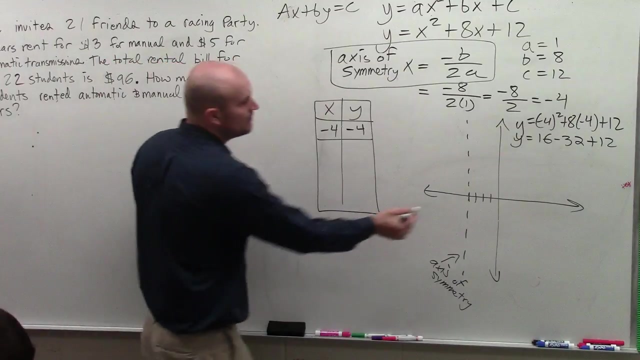 And I get: y equals 16 minus 32 plus 12,, which is negative 16,, negative 4.. Right, So now I go left- negative 4 and I go down negative 4.. 1,, 2,, 3,, 4.. 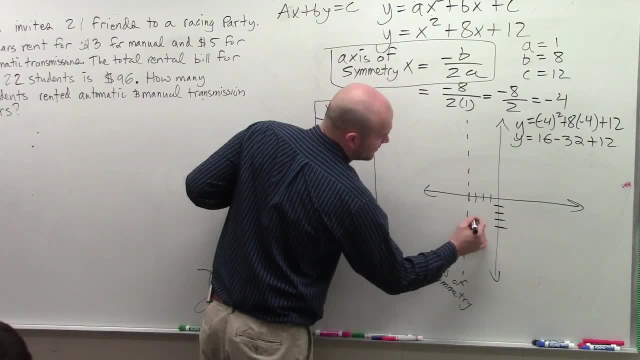 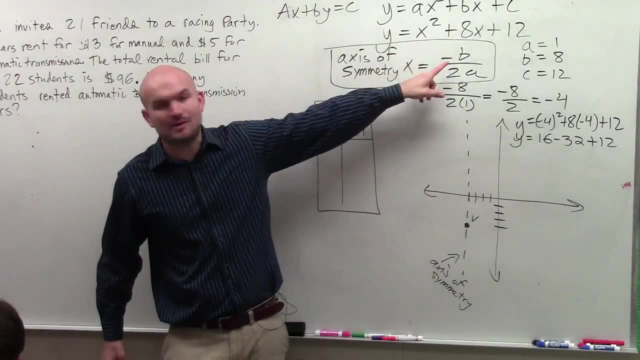 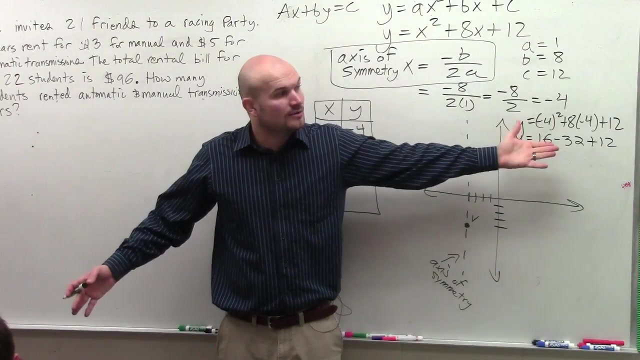 And that is now my vertex. What's necessary? All you've done is do opposite of b divided by 2a. You found that value and then you plug it back into the equation. Okay, Now let's pick. We need to pick two more points. as I mentioned, We need to pick two points to the left or two points to 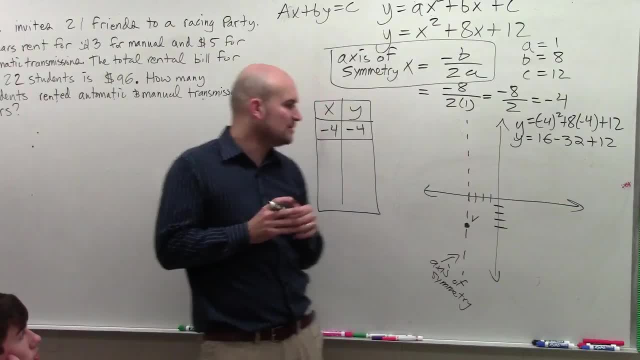 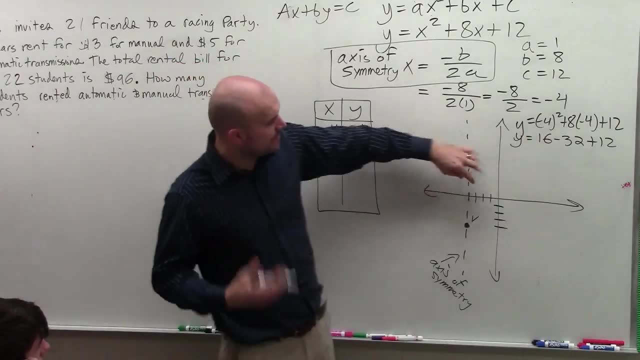 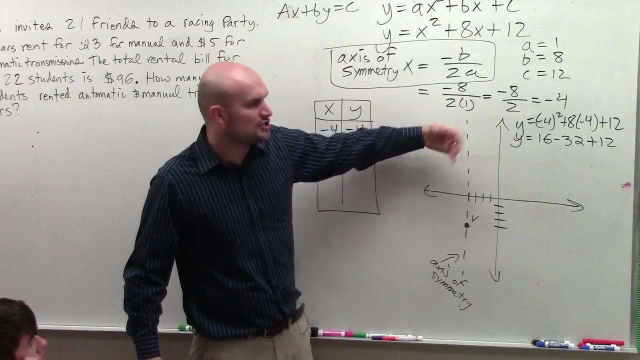 the right. What would you like to do? Pick two points to the left or to the right, To the left. Well, my recommendation would always be smaller numbers, right? It's much easier to pick numbers that are smaller than going larger. I mean larger in like absolute value, right? So let's just do. 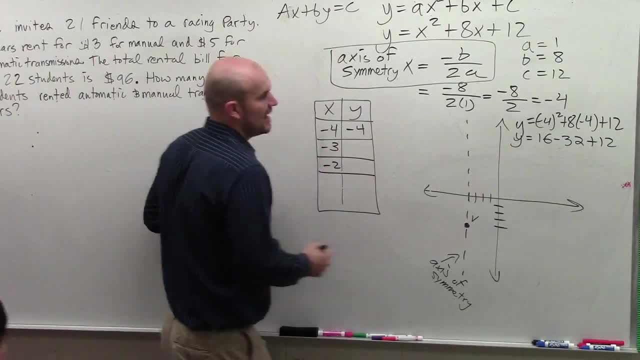 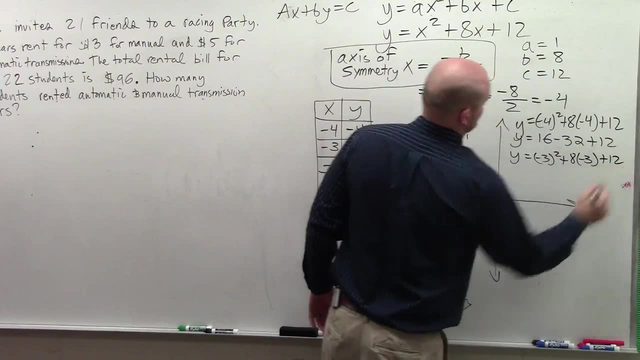 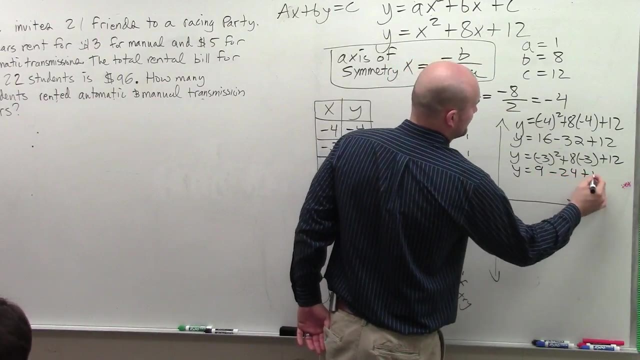 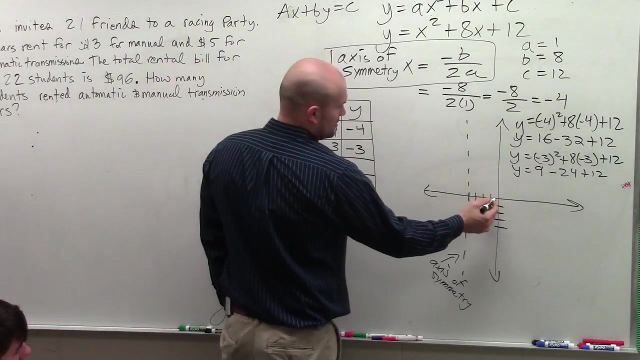 to the right. So now I'll do negative 3. When doing that, I get: y equals 9 minus 24.. Plus 12. That becomes negative 12, 9. That becomes negative 3. So that becomes negative 3,.